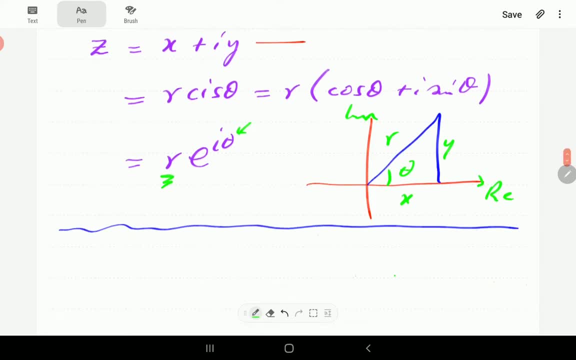 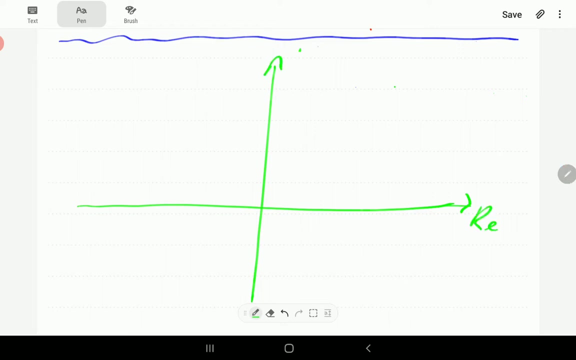 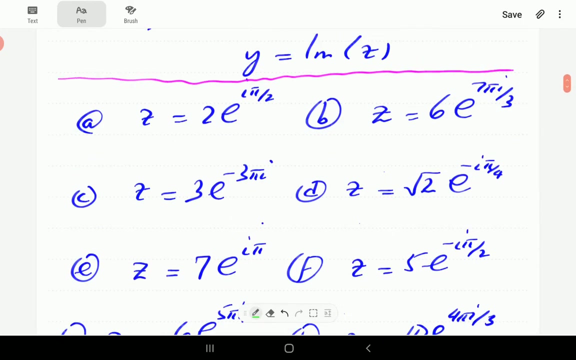 real axis. all right, so um, we're just going to start with the plotting um. so we're going to try and plot first three numbers. so if this is our arcane diagram, so first we have got z equals to 2e to the i pi on two um. so the thing we're going to do, 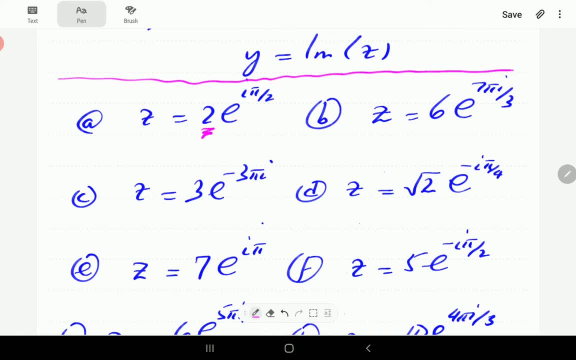 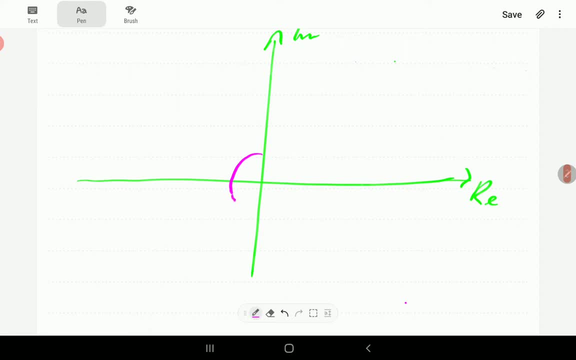 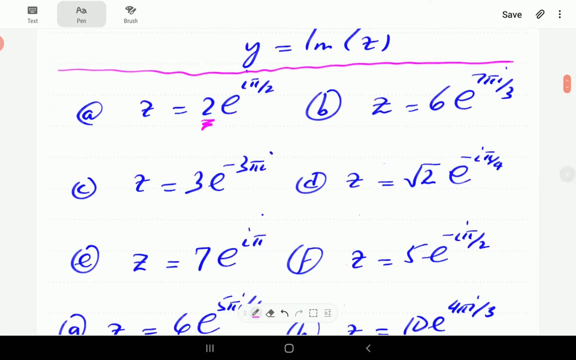 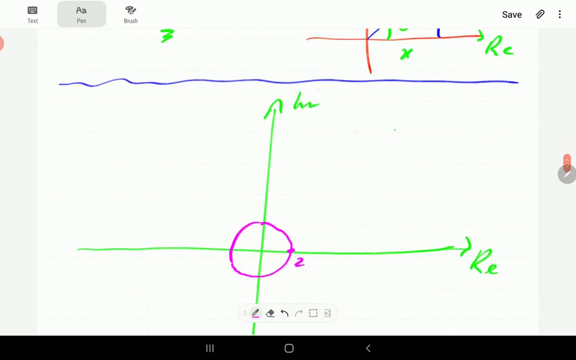 is uh. so from here the radial distance from the origin is two. so i'm just going to make a circle of radius two here. okay, so that's going to be two, so the complex number is going to be on that circle. but then the um, the argument is pi on two. so maybe, um, let's uh, uh, just uh, talk about what the 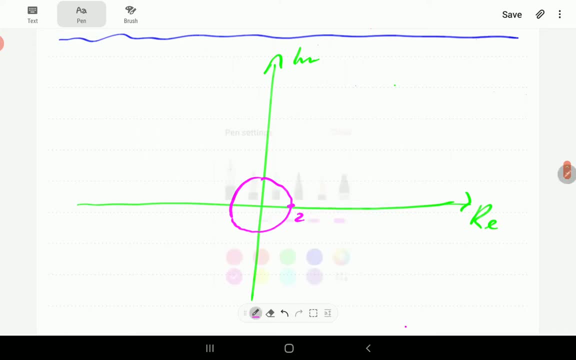 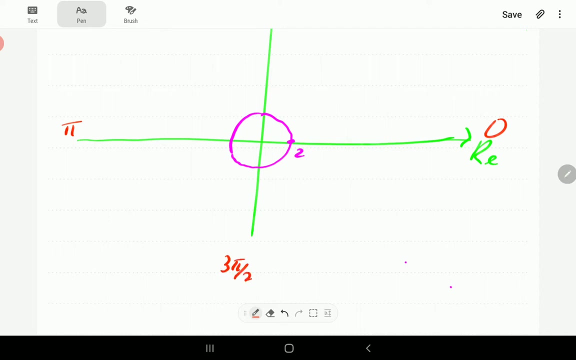 arguments are on the x's um. so starting um here, obviously this is zero degrees. this one is going to be 90 or pi on two, and then here this is going to be 180 or pi, and then here this is going to be 270 or 3 pi on 2, and then, coming back to the positive real axis, that's going to be 2 pi. 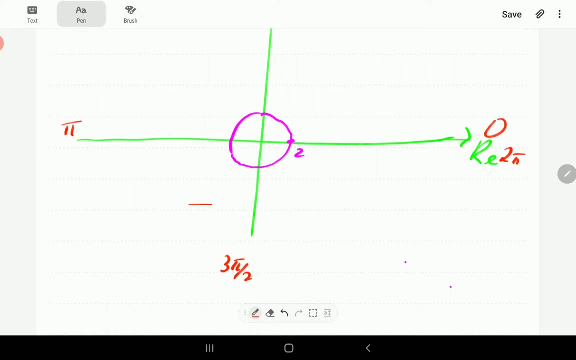 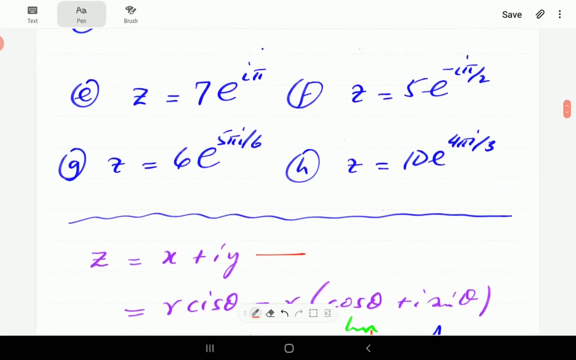 then if we go the clockwise root, 3, pi over 2 is going to be the same as negative pi over 2 and pi is going to be the same as negative pi. so we're just going to keep those ones in mind. so the for the first complex number. 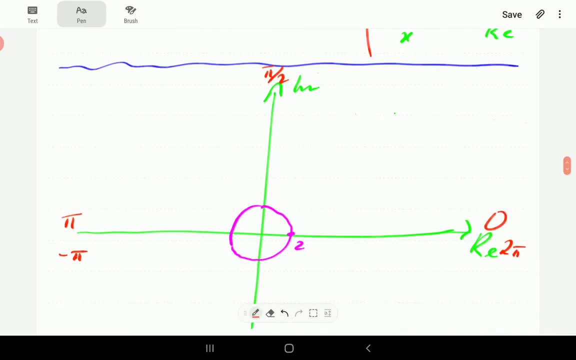 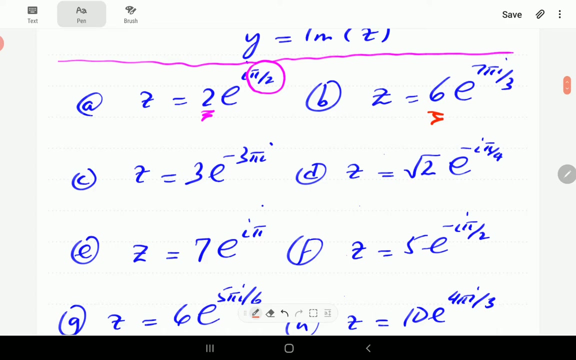 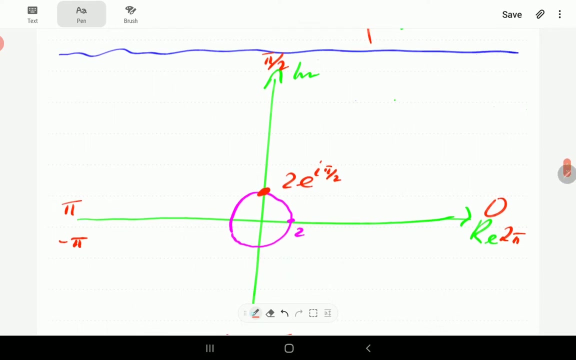 the argument is pi over 2, so that means this number is going to be located here. 2e to the i: pi over 2, so that's where that number is going to be located. the second number, the radial distance, is 6, so we're going to have to sketch a bigger circle, so suppose this is our. 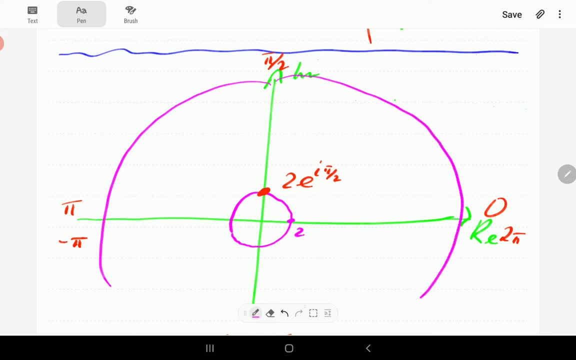 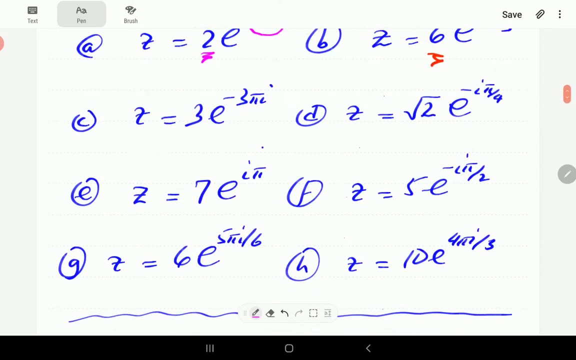 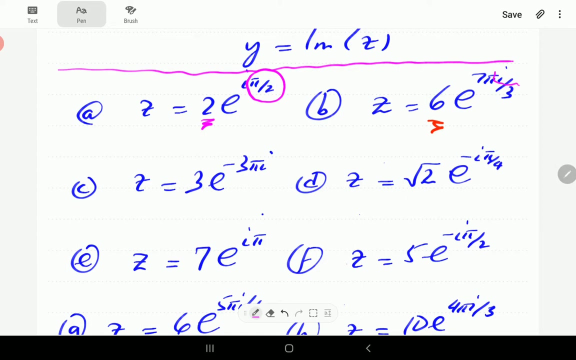 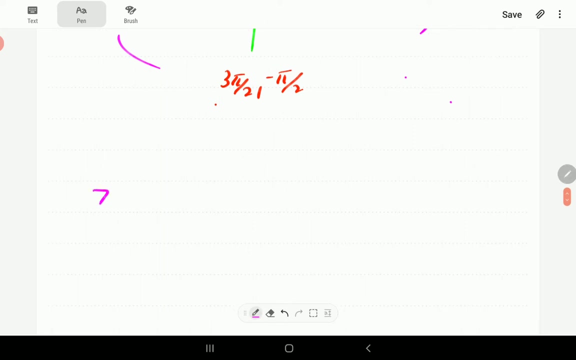 uh, bigger circle, and imagine that this is 6 there, so the complex number is going to be on that circle. then here we've got 7 pi over 3 as our argument. 7 pi over 3- uh, maybe just we're going to work this out here. 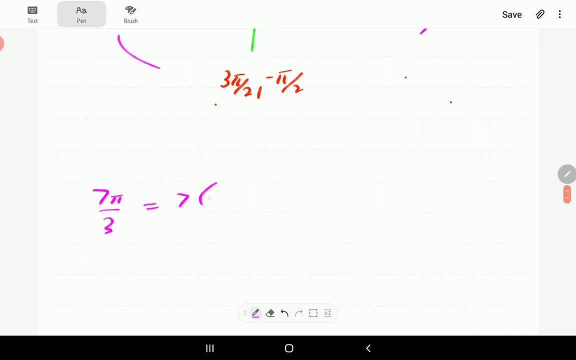 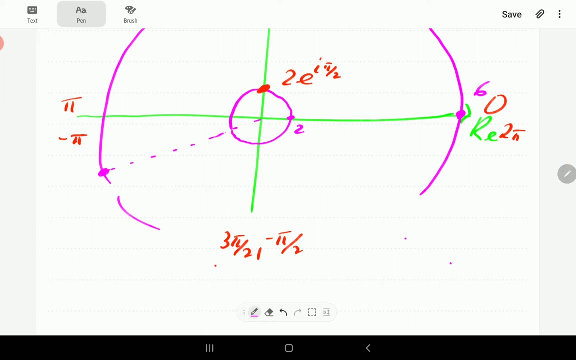 um, so so. so in degrees this is 7 times 180. then divided by 3, 1, 8 over 3 is 60 times 7. so this is going to be 210 degrees. so this complex number is going to be located there. so the distance from the origin. 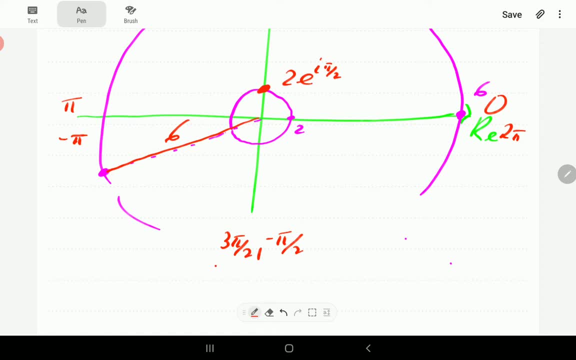 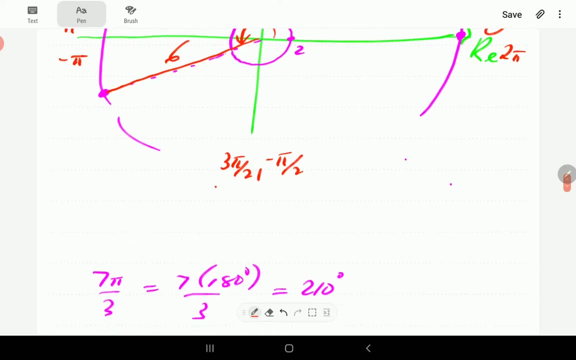 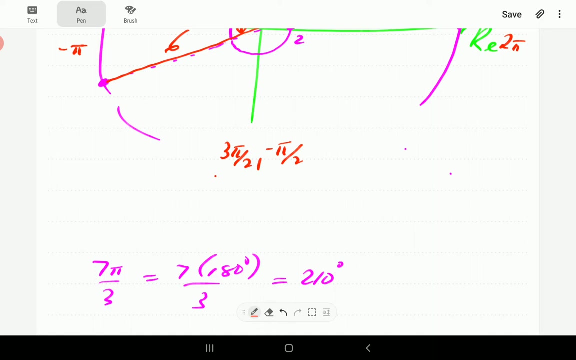 is 6 v. the angle here is 210 degrees, or 7 pi over. okay, that doesn't look correct. 7 times 6 is going to be actually what is 7 times 6? 7 times 6 is going to be 420. uh, then we're going to have to do this again. 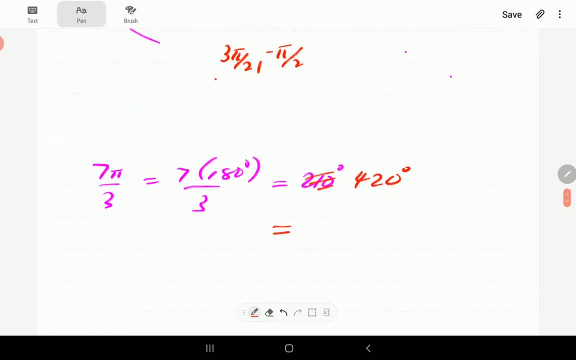 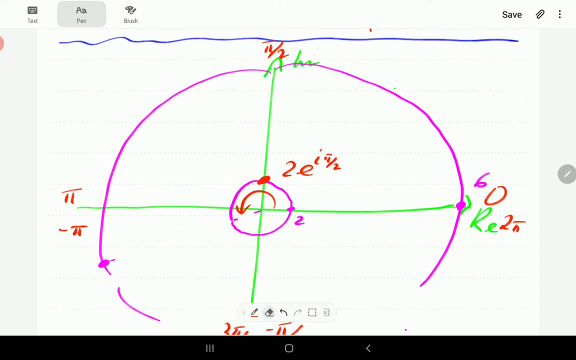 about when. when the angle is bigger than 360, then when the angle is bigger than 360, you take away 360. so for 20 minus 360 is actually 60. so this complex number is in actual effect, going to be in the first quadrant. 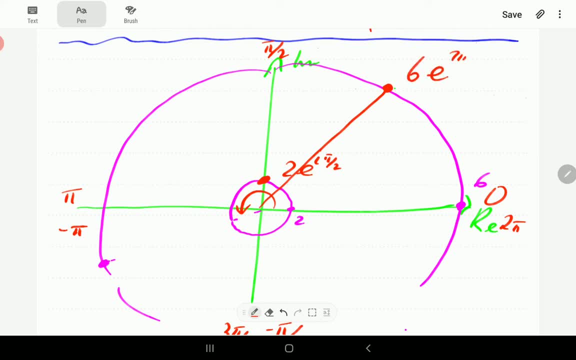 at 60 degrees. so there you are. so that's going to be 6e to the 7 pi over 8.. Wal, because that is this angle that I'm going to use here for the representation: seven pi i over three. that distance is six there. this angle here is seven pi over three. 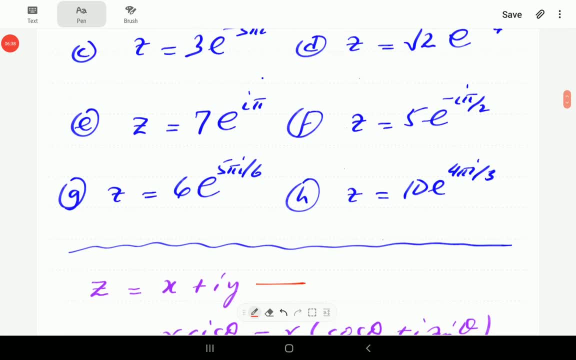 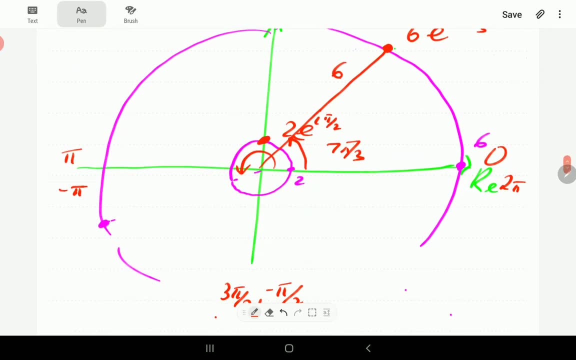 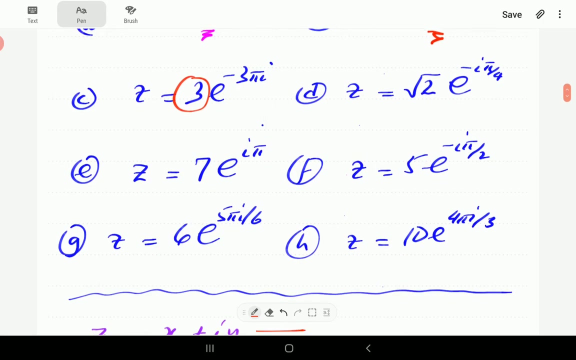 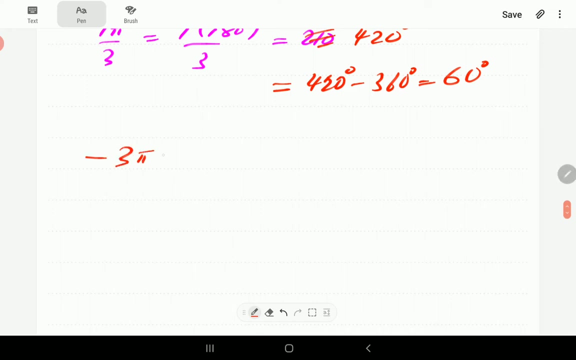 so that is the second one. then if we go to the third one, radial distance is three, so we're going to have to. we just do another circle here. the circle is of radius three, then the angle is negative three pi. so negative three pi is the same as negative three times. 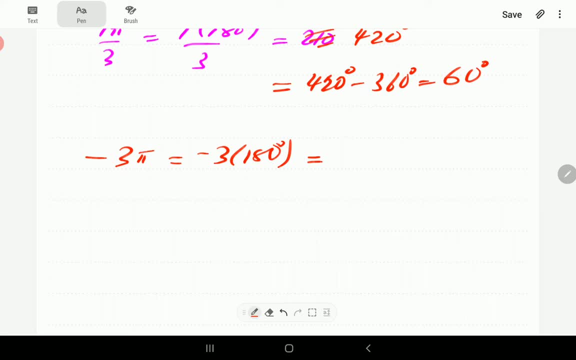 a hundred and eighty, so that is going to be three times eight is 24, so that's going to be negative 540. and so again, when this happens, we take away a multiple of 360.. so if we add 360 to this, so negative 540. 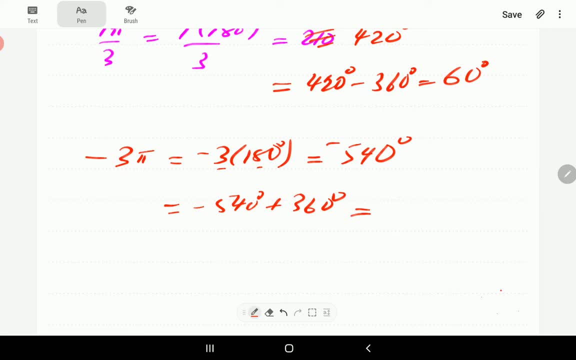 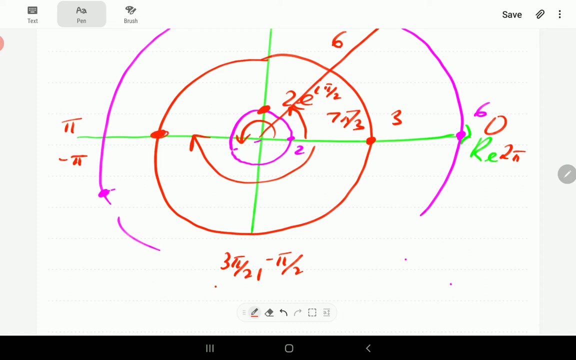 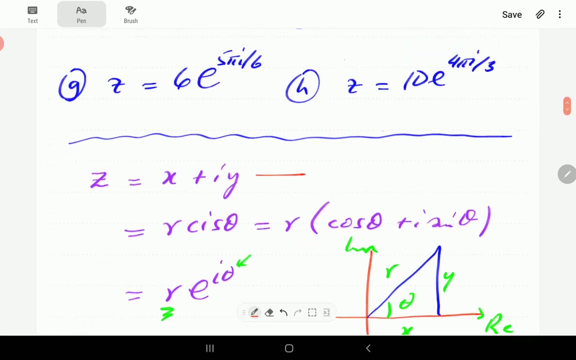 plus 360, then we're going to find that this is negative a hundred and eighty. okay. now, negative 180 is simply that angle there. so that means our complex number is going to be located there. so that is 3e to the minus 3i pi. okay, and then for the fourth one. 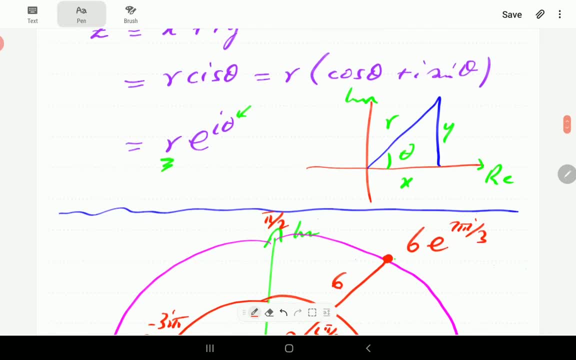 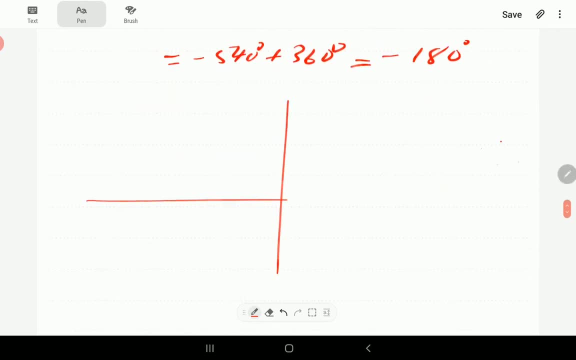 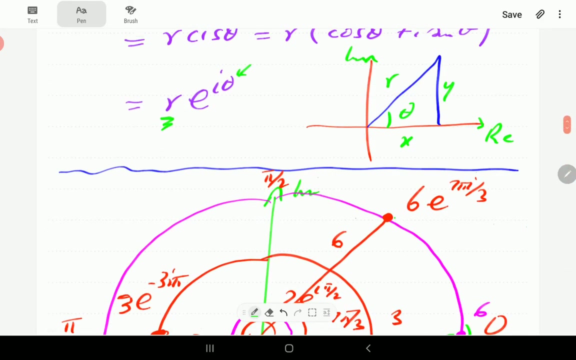 uh, the radial distance is root two, um, so maybe let's do a different sketch here. so this one: the radial distance is root two. so just going to um, take this circle in my chain, that is root two there and then the argument is negative. pi on four. 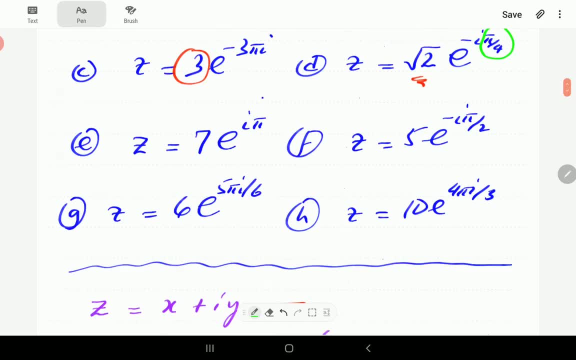 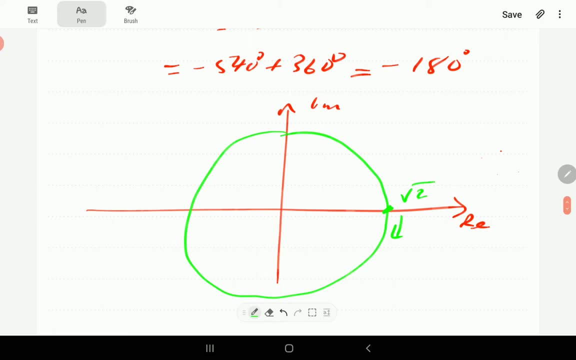 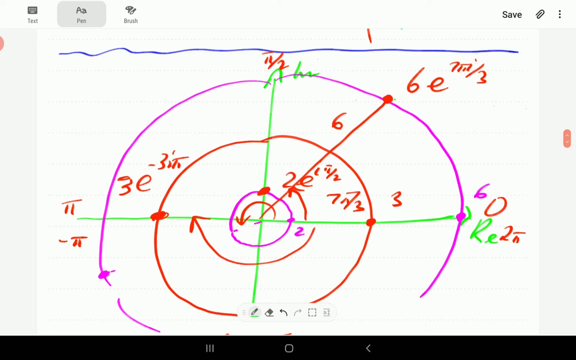 okay, negative pi on four. so that means going from the positive real axis, we're going to be going in the clockwise direction. pi on 4 is 45, so this one is going to be right here. so that's going to be root 2e to the minus i pi on 4.. so that's going to be those first four numbers, if we plot them in the 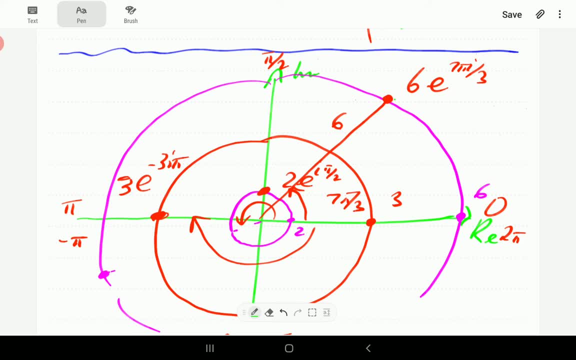 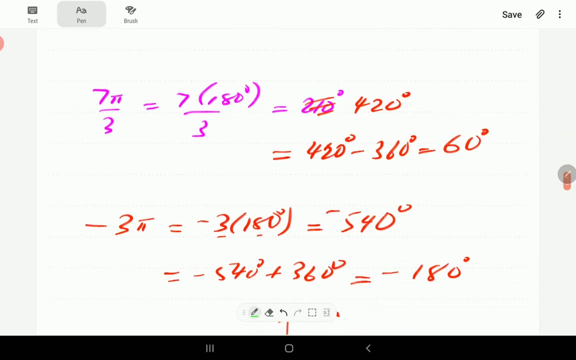 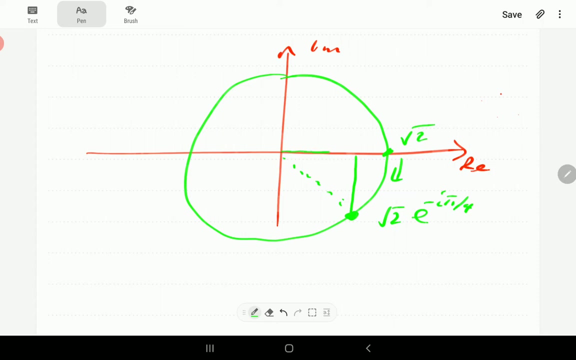 right direction. we're going to get the second diagram now, so notice that, uh, in terms of the exponential form, all that matters is the radial distance from the origin and then also the angle. then, when we start expressing these numbers in rectangular form, then we ask ourselves the question: 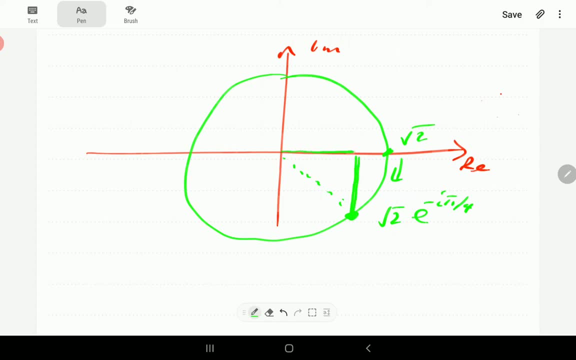 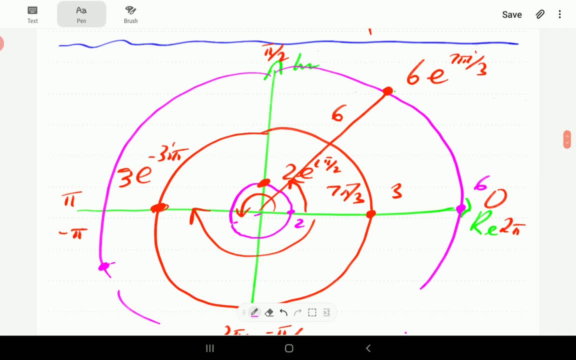 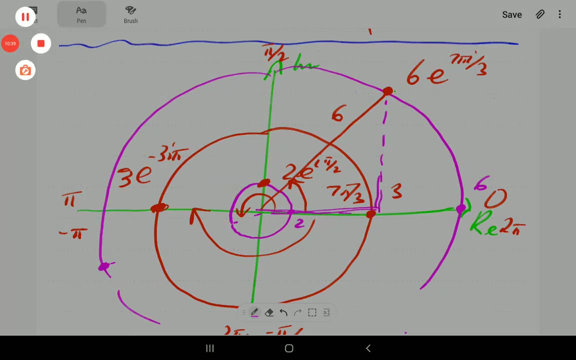 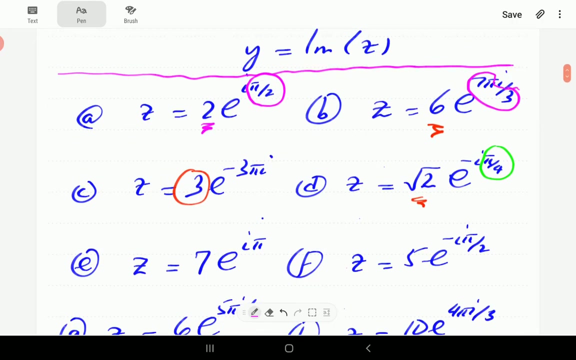 and then for each of these, that's exactly, uh, what we're going to do. so for this one, for instance, it's going to be a real, uh, your imaginary component, and that is going to be the real component. okay, um, now. so the question is: how do we then find the rectangular form? 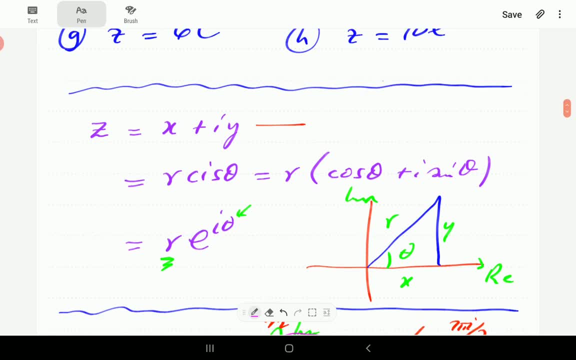 given the complex number in exponential form. so how do we go from this form back to this form? the answer is we go back to that form via the polar form. so from there we express things in polar form and then, once it's in polar form, we've already seen.